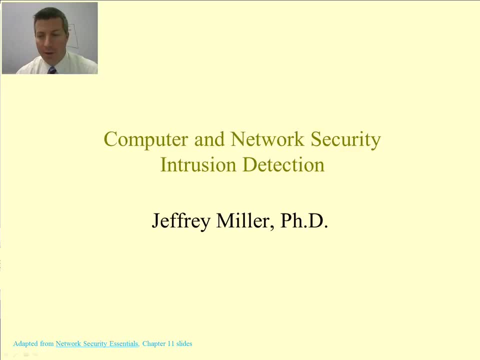 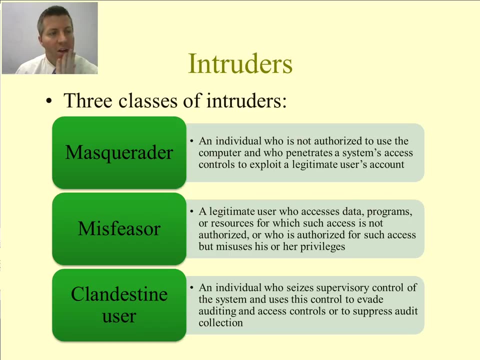 Welcome to Computer and Network Security. Today, our topic is on Intrusion Detection. Okay, so one of the two most publicized threats to security is an intruder, with the other one being something we already talked about, which is viruses. Intruders are often called hackers, and there are three different classes of intruders. The 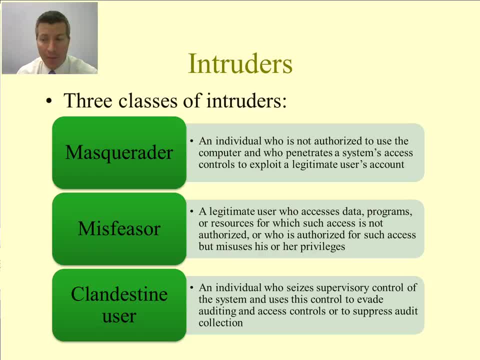 first one is: a masquerader: an individual who is not authorized to use the computer and then penetrates a system's access controls to exploit a legitimate user's account. A misfeasor: a legitimate user who accesses data, programs or resources for which access is not authorized. 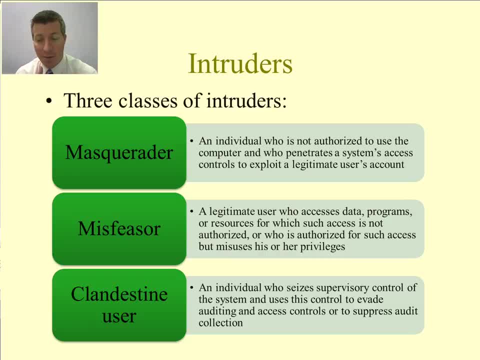 or who is authorized for such access but misuses his or her privileges. And then the clandestine user, an individual who seizes supervisory control of the system and uses this control to evade auditing and access controls or suppress audit collection. The masquerader is likely to be 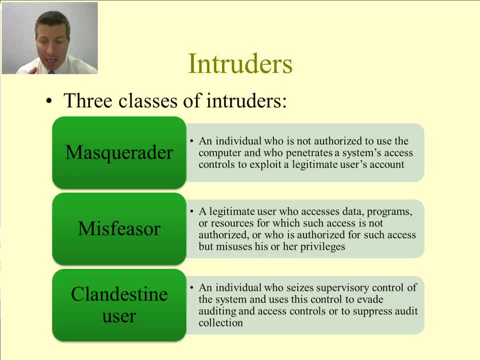 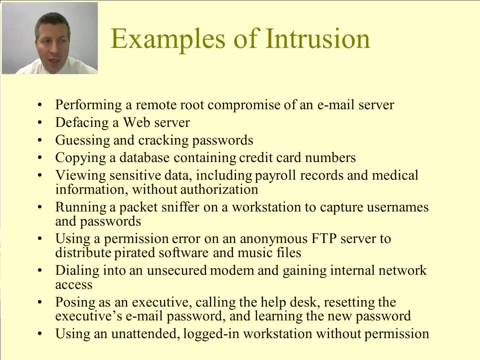 an outsider. The misfeasor is usually not. Actually, the misfeasor is usually an insider, and then the clandestine user is going to be could be either from the inside or the outside. Here are just some examples of intrusion. They range from being benign. 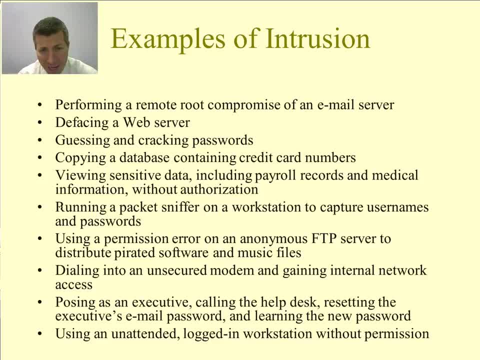 to being serious. So, at the benign end of the scale, many people just wish to explore the internet and see what's out there, and they may not even be trying to intrude. On the other hand, the more serious intruders are going to try to read privileged data, perform some unauthorized 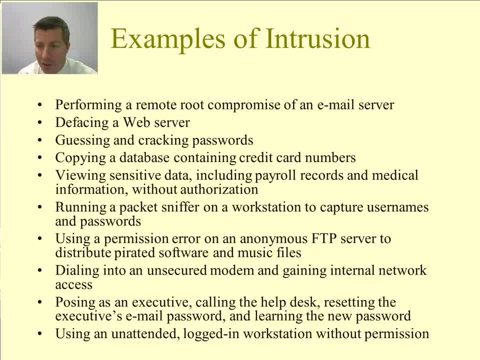 modifications to data, disrupt the system and so on. So you can see some examples here of intrusion, messing in, cracking passwords. So that could be benign or it could be very malicious, depending on what the intent is behind that: Copying a database containing credit card. 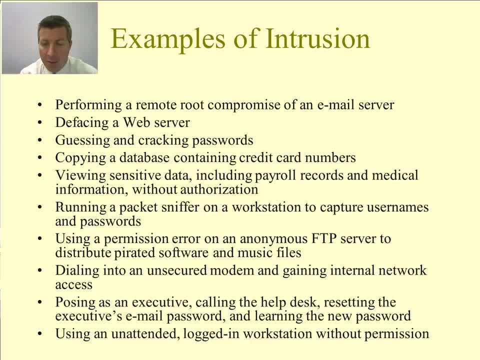 numbers. most likely, Most likely that one is going to be malicious Running a packet sniffer on a workstation. That one by itself could be benign, but if you're trying to capture usernames and passwords for people who log into it, obviously, then it's probably getting. 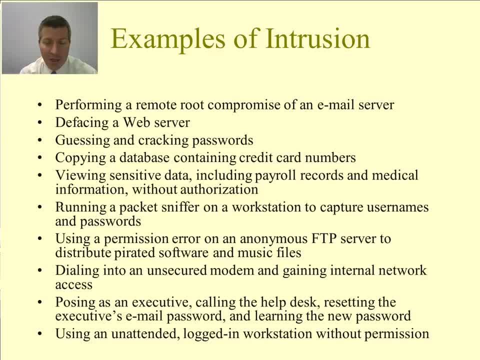 more malicious Dialing into an unsecured modem, gaining internal network access. These are all issues that possibly network security experts would want to test on their own networks. However, if you're doing this in a malicious manner or on a different network, then this is going to most likely a lot of these. 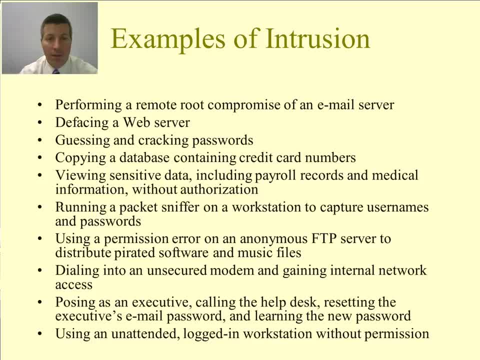 things would be deemed illegal. even So, make sure that you understand. if you're trying to do any of this and you're just trying to protect your own network is one thing, but depending on how you use the data or what the purpose of you doing that is, it might be deemed illegal. 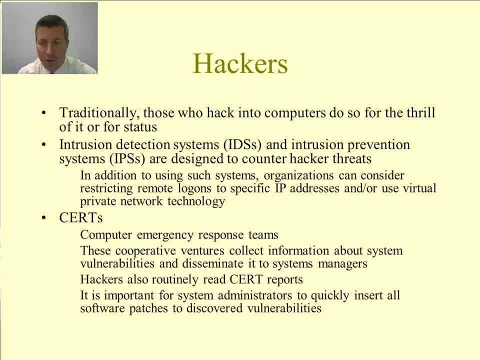 So a hacker- traditionally those who hack into computers just do it for the thrill or for status. A lot of people that hack they're not necessarily trying to get any financial gain out of hacking. Some people are, but the majority of them do it just because they. 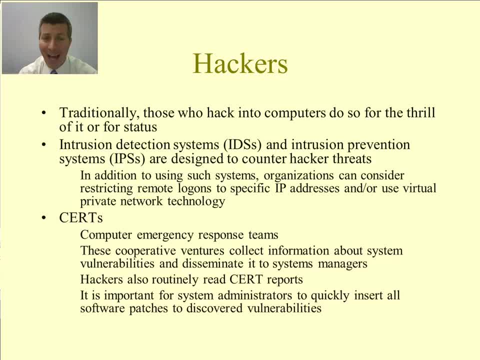 want to see if they can. These are typically very, very smart people and it's sad that this is how they're using their abilities, because they are very intelligent And if they are able to hack successfully, then they probably had some other career path in mind that they could have made a lot. 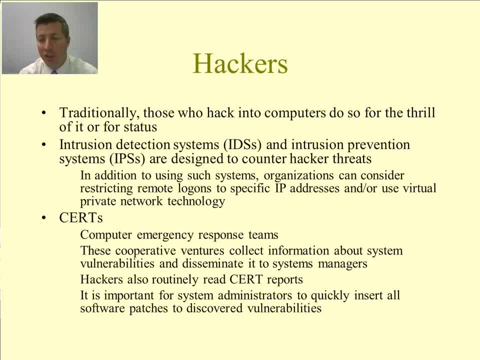 of money on rather than just being a hacker. But so a lot of people do it just to see if they can. Intrusion detection systems- IDSs, and intrusion prevention systems, IPSs, are designed to counter the hackers, the hacker threats. So organizations can consider also restricting remote logons. 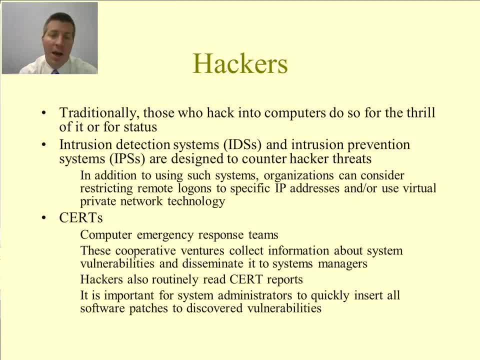 so specific IP addresses, use virtual private networks and so on. These are just some of the technologies which try to circumvent hacking into it. A lot of organizations have what are called CERTs. These are Computer Emergency Response Teams And what they do is just to monitor the network. Hackers often will read CERT reports because 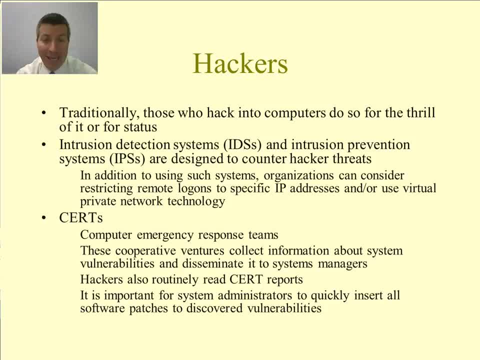 that's going to give them a little bit of insight. A lot of those reports might be internal and so these could be internal hackers if they have access to them, And it's important for system administrators that you have to make sure that you keep. 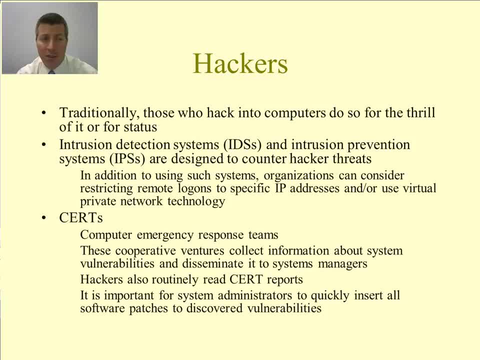 all of your patches up to date. It's really hard in large corporations to make sure this happens, which is why they have, first of all, more network administrators, security experts, in the company, But they also have more problems because it's hard for them to. 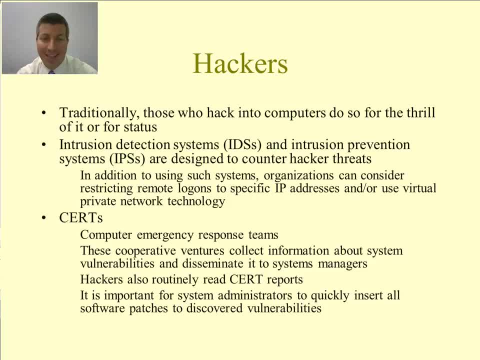 systematically make sure that every single computer in the organization gets the correct update, the correct patches. Especially if you have a lot of different applications that are running in different departments and so on, you have to make sure that they all mesh and that they're not going to have any problems from it. So that's very difficult, But it's. 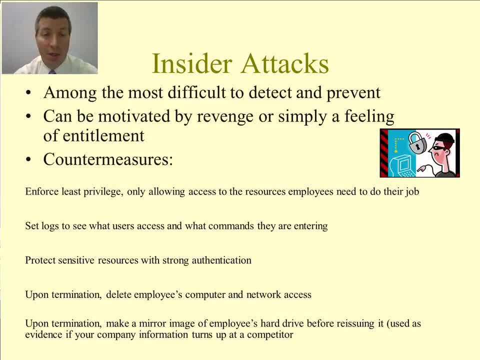 very difficult for a lot of companies and corporations, organizations, to do. Insider attacks are by far the most difficult to detect and prevent because that user most likely already has some kind of access that outside users probably do not have, So it makes it a lot harder to find them out. It can be motivated by revenge. 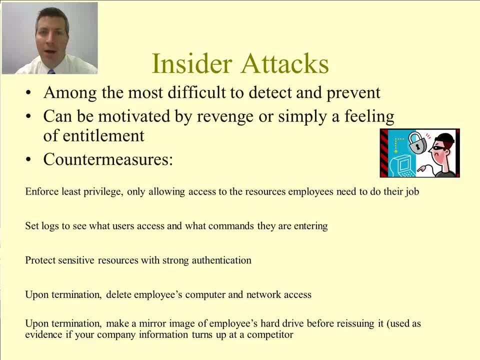 Maybe this is one reason why, when IT personnel are let go, either laid off or fired, they often are not given notice And, as soon as it happens, all of their privileges are taken away, their keys are taken away and they're escorted out of the organization. This is because they 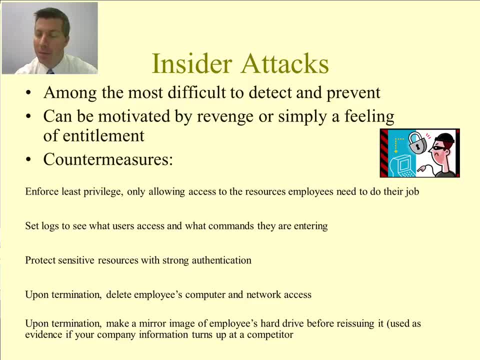 have a lot of authority, typically, or more so than other people, and they could really really hurt the company. Now, it would be illegal if it was malicious. However, the company would still have to try to recover somehow, And so it's easier if you just don't. 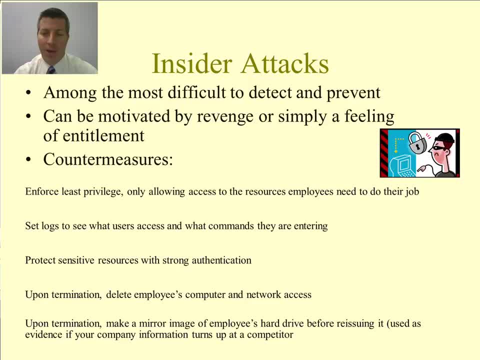 let the situation arise. Don't put yourself in the situation where that could potentially happen. Some countermeasures Organizations do not want to give people root access. You want to give them the least privileges that they need. You don't want to give them more than they actually need. 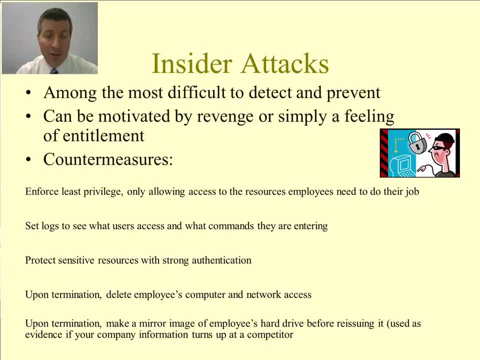 to do their job. If you give them more than that, then you're setting yourself up- The company at least, is setting itself up- for possibly having something happen. Set logs so you can see what users access what commands they are entering. This is very, very easy to do on many operating. 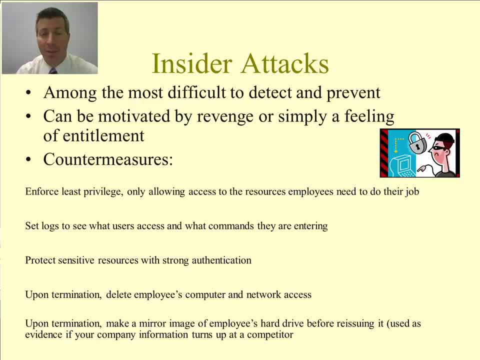 systems. Linux has it, where you can track and see absolutely every single command That a user runs, and it'll store it into a file, So that would probably be something good to do. Protect sensitive resources with strong authentication, So make sure that not very many people have. 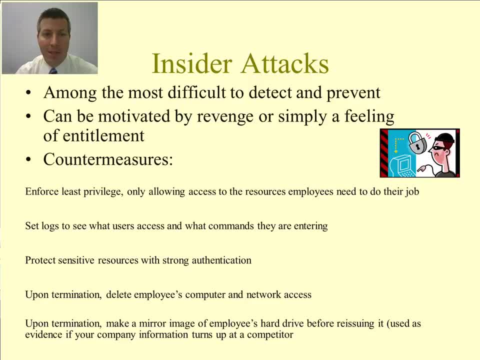 it, if any, and make sure that the authentication is very strong, that it's not based on some dictionary word. Upon termination, delete the employee's computer and network access. This usually happens during the termination, So as soon as it's decided, this person is. 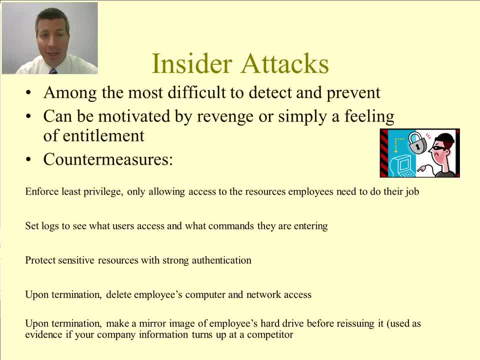 going to be terminated. while they are in talking with their manager or bosses, the other people are actually deleting all of their access, Possibly wiping their hard drive and just getting rid of everything that they have, Assuming everything's been passed off and backed up somewhere. 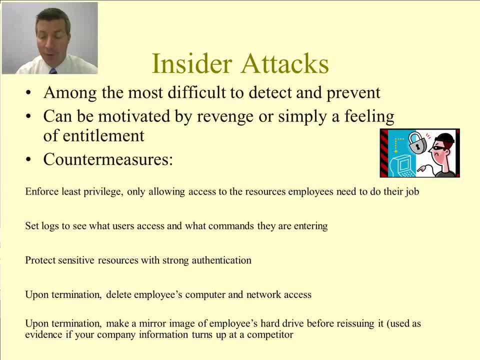 Upon termination, make a mirror image of the employee's hard drive before re-issuing it. Use as evidence if your company information turns up at a competitor. So this is very, very important Also, that you make sure that you've made a mirror image of the 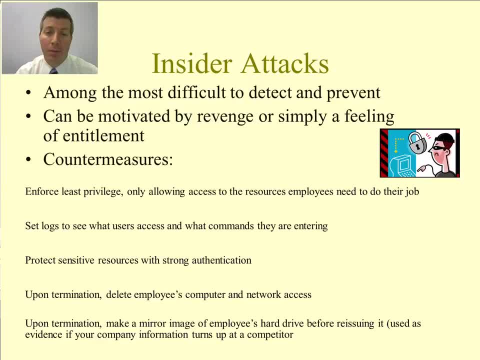 employee's hard drive and then, chances are, what you're going to do is you're going to probably just wipe that drive, install a fresh new installation. That's a real clear violation of the operating system on it, but you want to make sure that. 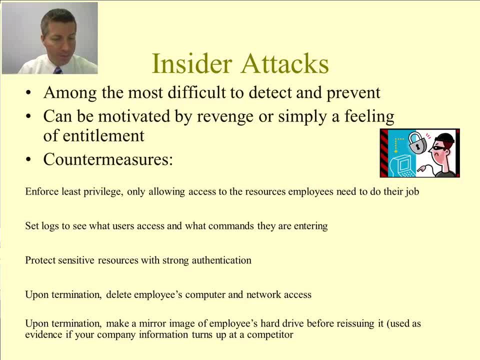 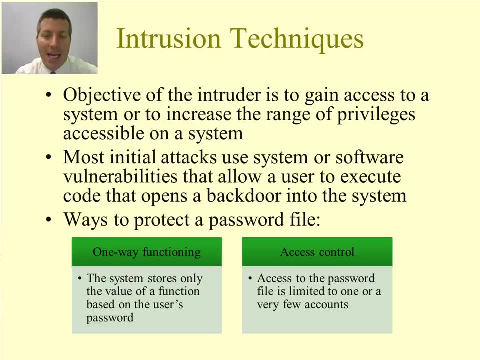 you keep that back up. as I just mentioned, Here are some intrusion techniques. First of all, the objective of an intruder is typically to gain access to a system or increase the range of privileges accessible on that system. So most initial attacks use system or software vulnerabilities that allow a user to execute. 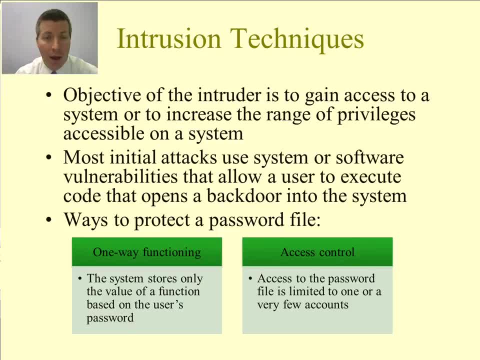 code that opens a backdoor into the system. One approach here: most organizations are going to have a password file. Now, typically this is not a file which is unencrypted, and the passwords themselves that are inside the file are typically not unencrypted. If that is the case, 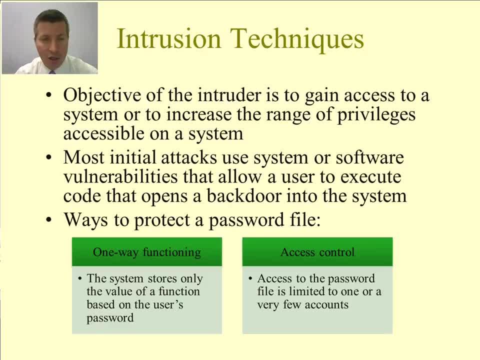 this is something that needs to change immediately. at an organization. You don't want to have unencrypted passwords just sitting on a server somewhere, So the passwords are typically encrypted, but all of the passwords are stored in a file. This is how Linux works. also, You have a. 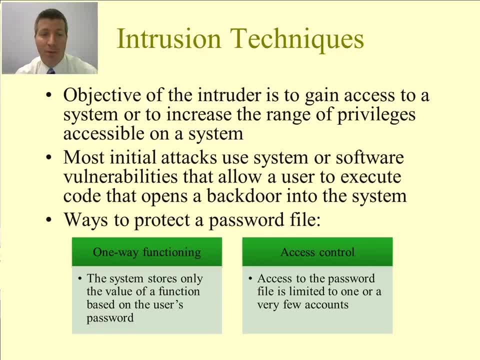 password file and inside of that you have these passwords that are encrypted. You probably want to protect that file. also. You don't want somebody going into that file and changing all of those passwords. If that were to happen, people wouldn't be able to log back in and try to fix things. 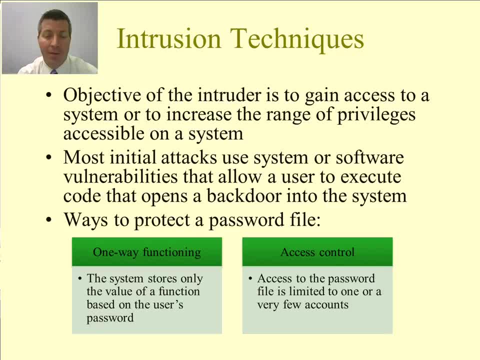 You would have to somehow have root access or be able to override whatever they change inside of that file. So it would be very good if that file had strong encryption on it. so it's very limited to one account or just very few accounts. That's the access control. 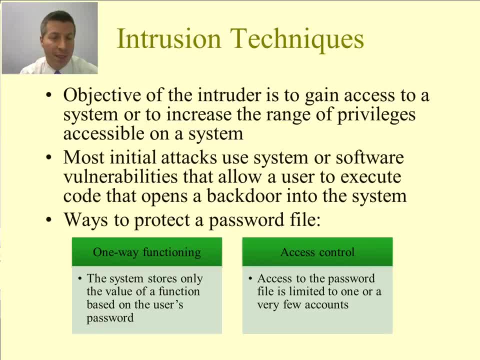 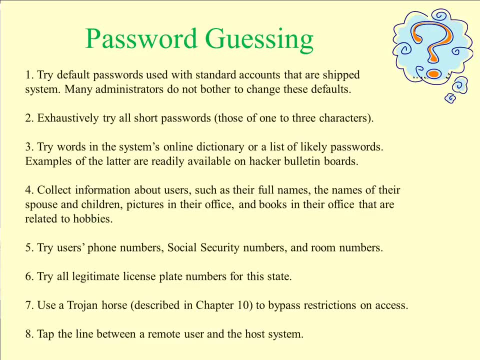 The one-way functioning. the system stores only the value of a function. basically It's based on the user's password. So those are two ways that you can hopefully fix that Password: guessing, If you want to just try to guess, and again, I don't tell you these things. 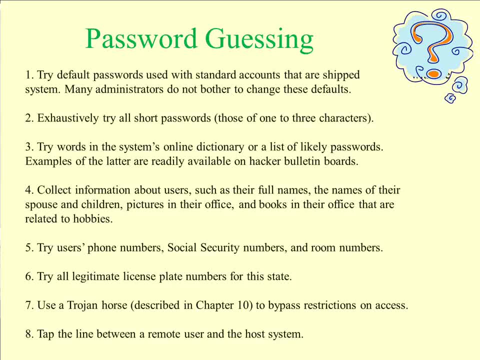 so that you can try this. I do this more so that you can figure out if your network is more secure. So here are just some strategies. if you're trying to guess a password, Try the default passwords with standard accounts that are shipped with the system. This would be like: 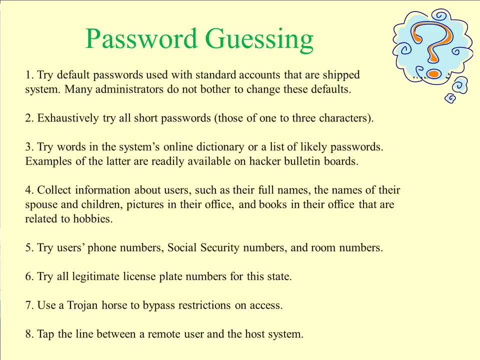 let's try admin. Let's try password. Let's try PW. Let's try no password. These are very, very common. You never want to have one of those passwords as the password on one of your accounts. A lot of wireless routers: people will buy a wireless router and they hook it up and it just 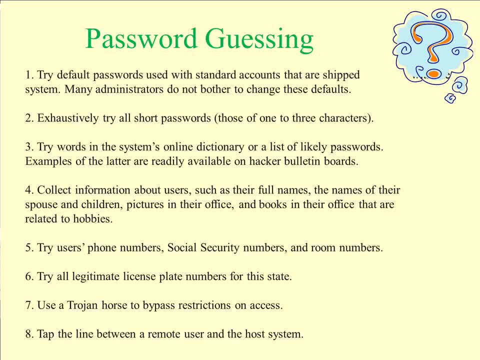 works right out of the box. It's really great that we have that. However, a lot of them have a default name of the wireless network as Linksys or Cisco, with a number following it, And then the admin passwords, maybe like admin for the username and admin for the password. You don't want to do that. You've got to make sure. 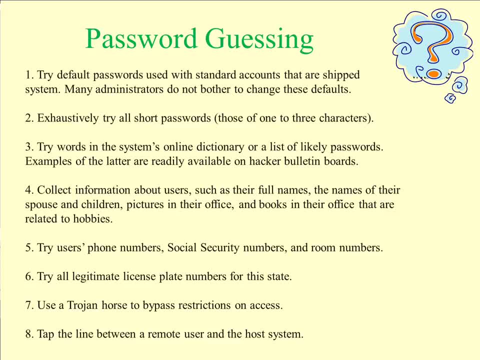 you go in there and change what that password is. You can exhaustively try all short passwords which are from one to three characters. Those are terrible passwords. You know that a lot of passwords require you to have at least eight characters. They want some combination of numbers. 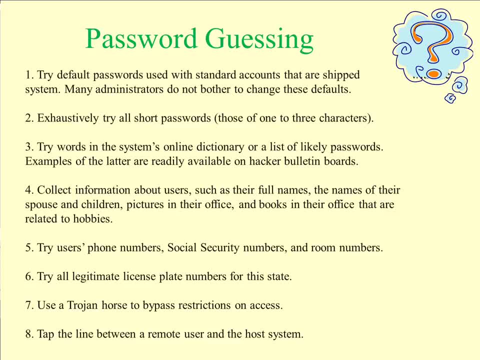 and characters possibly, or letters, possibly, even some symbols that have to be in them. Those are going to be the best ones. They're typically not based on dictionary words, because there are programs which just go through all of the words that are in a dictionary. 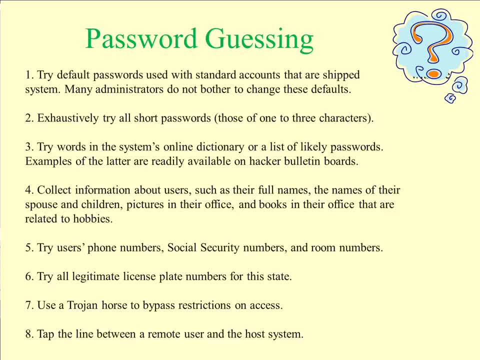 and try each one of them sequentially. And that's number three. Try the words in a systems online dictionary or a list of likely passwords. You can find these online. Collect information about users. This one's getting a little bit more sophisticated. If you know a user's full, 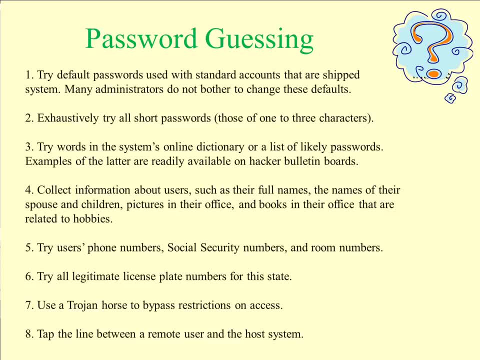 name. you know the names of a user's spouse and children. Oftentimes people will use those as their passwords. Look at what pictures they have in their office books in their office that are related to hobbies. These are some strategies that could be used. These 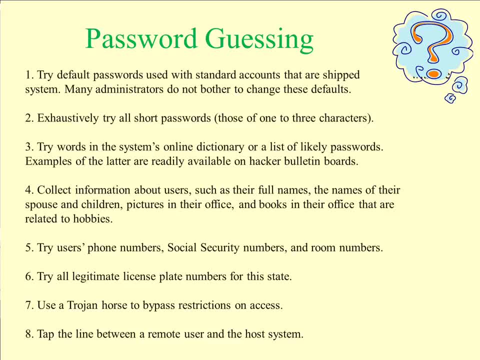 are probably. if you want to have a really good password, don't base it on any of those things. Phone numbers, social security numbers, room numbers, addresses, license plate numbers- These are not things that you want to base it on, because these are things that can be. 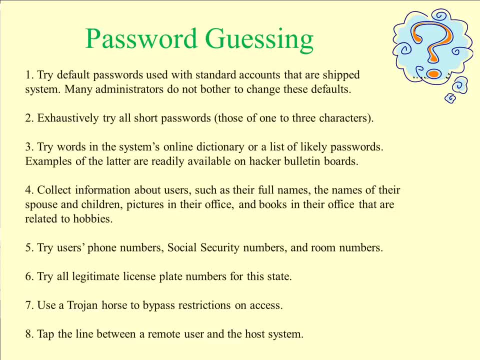 tied back to you somehow, So you want to make sure your password is not based on those things. I know a lot of you might be thinking: oh my gosh, I need to go change some of my passwords. Use a Trojan horse to bypass restrictions on access. We've talked about Trojan horses. 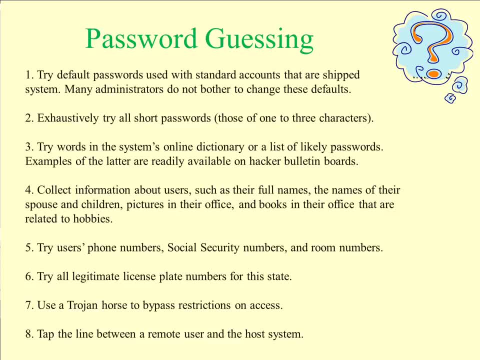 and how they can get around some security. Tap the line between a remote user and the host system. This would be something like a man in the middle attack. You can try to find out what the passwords are. This might not work very well because a lot of passwords are going to be encrypted between the host. 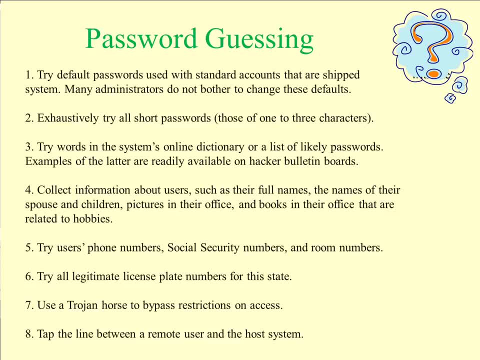 and the server. However, something else which is not on this list could be possibly using key loggers. That's not guessing a password, but on the other hand, that is one way that you could get it if you had a key logger installed on a computer. 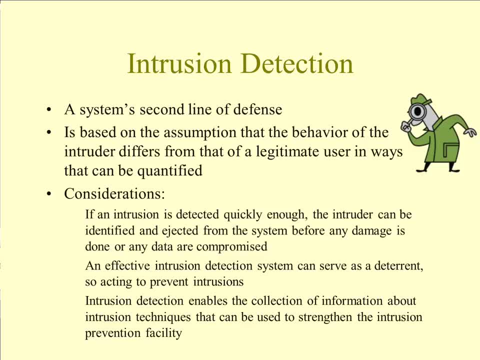 Okay, so specifically with intrusion detection. now, intrusion detection is a system's second line of defense. It's based on the assumption that the behavior of the intruder differs from that of a legitimate user in ways that, hopefully, can be quantified. So here are some. 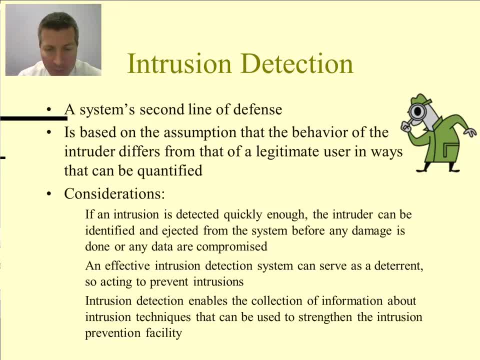 considerations that you have here. If an intrusion is detected quickly enough, the intruder can be identified, ejected from the system before any damage is done. An effective intrusion detection system can serve as a deterrent, kind of like having security systems on your home If somebody wants to get into your home, even if you have 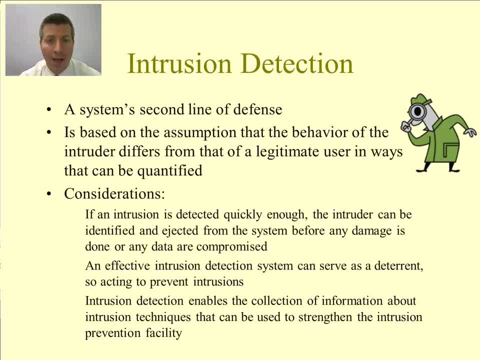 a security system, they're still going to be able to break a window or knock down the door and get in. However, the alarm is going to go off as soon as that happens. Security systems often work more as a deterrent mechanism rather than a countermeasure. So if you're 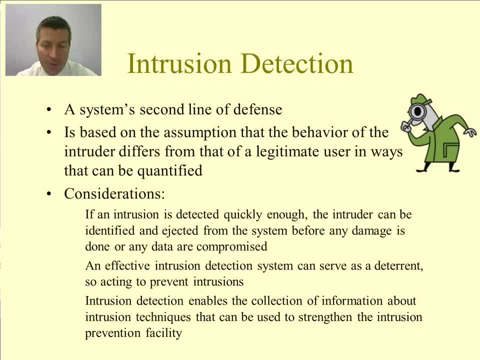 catching somebody once it happens. I mean that's secondary, That's the second line of defense. You're hoping that the security system and you've got that little sign out in front of your house or on your window that says that your house is secured, that that's going. 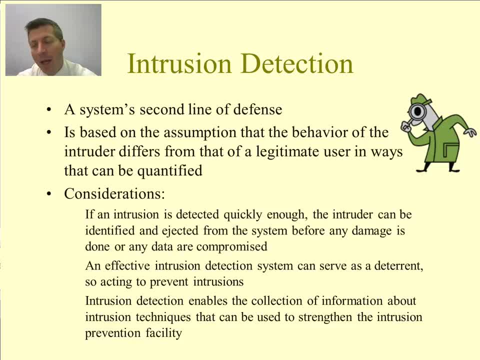 to be enough to deter somebody from coming into your home, and they'll probably look for an easier target rather than yours, And that's what an intrusion detection system hopefully will do also, And it also enables the collection of information about intrusion techniques that can be used then to strengthen future intrusion protection. 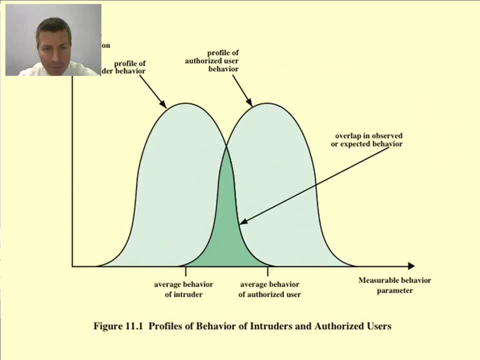 Okay, taking a look at this, this is just showing the profile of authorized behavior compared to intruder behavior, probability, density, function. So whatever these lines happen to be measuring here, the bottom line is that you're going to have some profile of what the network traffic looks like when you have authorized users on your network. 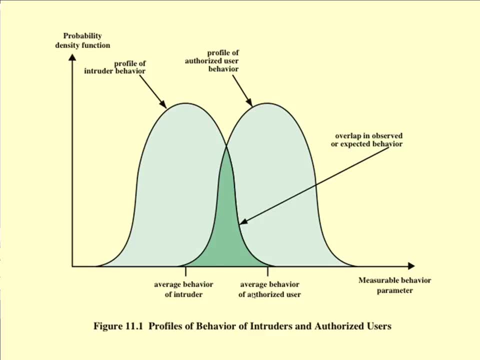 Then you're going to have a different profile. if it's an intruder, You have some overlap, and if the intruder is very sophisticated, they may be able to just operate in the area down here where you aren't going to be able to detect that it. 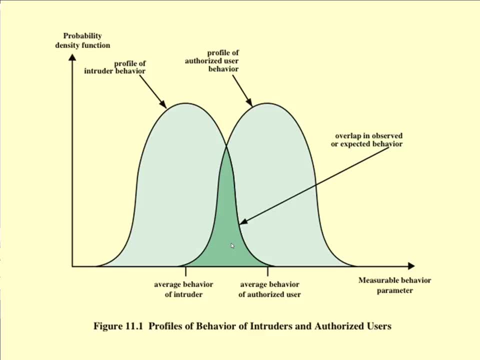 is an intruder that it looks like it could be authorized behavior. Many intrusions aren't like that and they're going to try to get as much as they can as quickly as they can, and that's where you're going to get this big spike right when it happens. 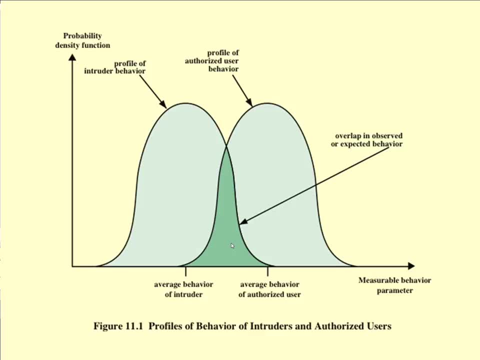 And so these types of graphs are often used. These are generated by intrusion detection systems. There would be computers that would just have these graphs on it constantly, throughout the day, and you have people monitoring it If there's some anomalous behavior that happens. 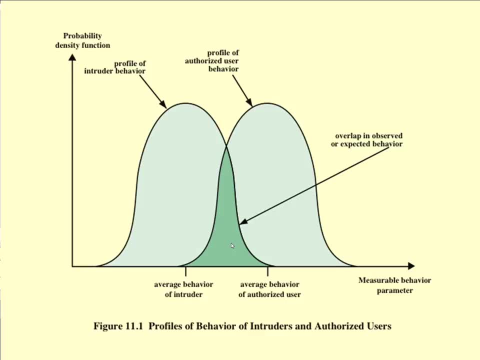 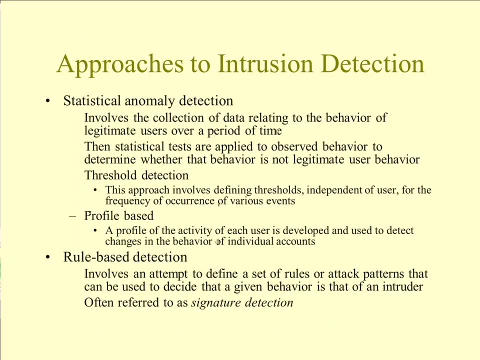 then it might send off an alert to some network administrators or system administrators that there's possibly some kind of an intrusion occurring right now. Some approaches that we have to: intrusion detection, statistical anomaly detection and rule-based detection. We'll go into these in a little bit more detail in the next few slides. 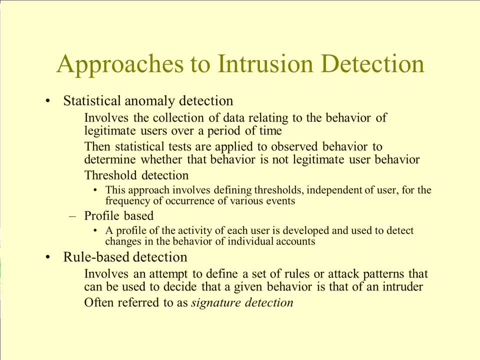 Statistical anomaly detection involves the collection of data relating to the behavior of legitimate users over a period of time. That's what we were just looking at on that previous slide. We determine with a high level of confidence in whether the behavior that we're currently seeing is legitimate or not, And there are pretty good algorithms for doing that already. 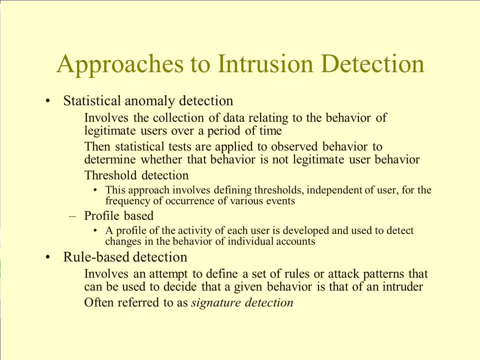 One of them is with the CALL. It's called threshold detection. This approach involves defining thresholds, independent of the user, for the frequency of occurrence of various events. The other one is profile-based: A profile of the activity of each user is developed and used to detect changes in the behavior of individual accounts. 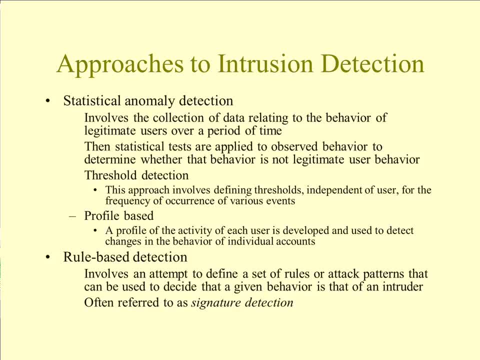 So, in essence, anomaly approaches attempt to define what's normal or expected, whereas the signature-based approach attempts to define proper behavior. Rule-based detection now involves an attempt to define a set of rules or attack patterns that can be used to decide that a given behavior is that of an intruder. 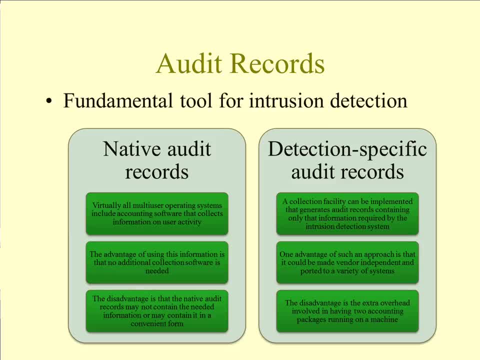 A fundamental tool that is used for intrusion detection is called an audit record. Some record of ongoing activity by users must be maintained for an intrusion detection system. There's two different ways that this input is fed into the intrusion detection system. One of them is through native audit records and the other is through detection-specific 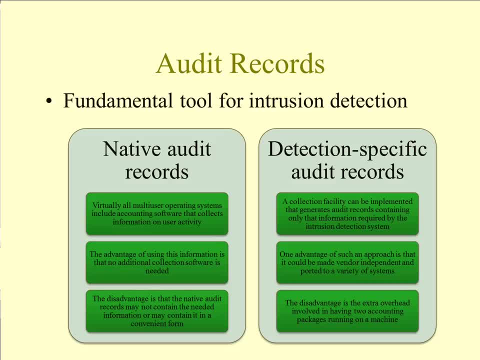 audit records With the native audit records. virtually all multi-user operating systems include accounting software that collects information on user activity. The advantage of using this information is that no additional collection software is needed, So we're able to see some information, Okay. 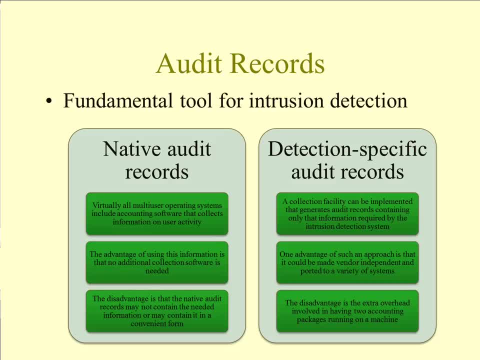 We're able to see information about user activity without having to install anything else on it. The disadvantage is that the native audit record may not contain the needed information or may not contain it in convenient form. So that's just a little disadvantage. You might need to mess around with the data a little bit to get it into the form that. 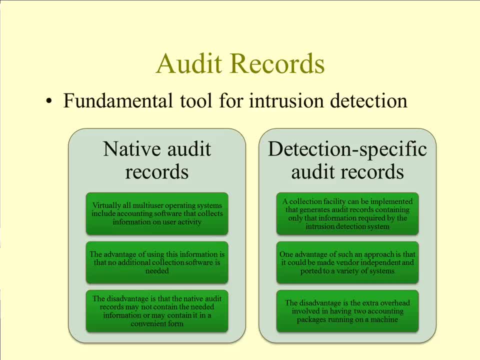 you need for your specific intrusion detection system- since this is going to be mostly built into the operating system of how it's detecting it- Detection-specific audit records. Now, on the other hand, a collection facility can be implemented that generates audit records containing only that information required by the intrusion detection system. 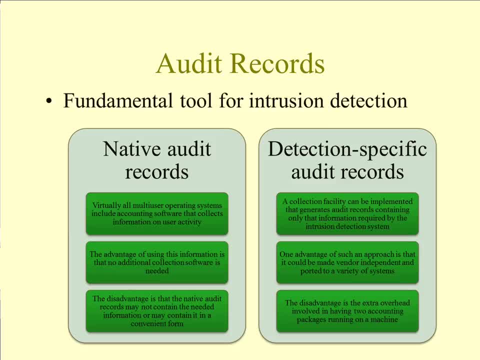 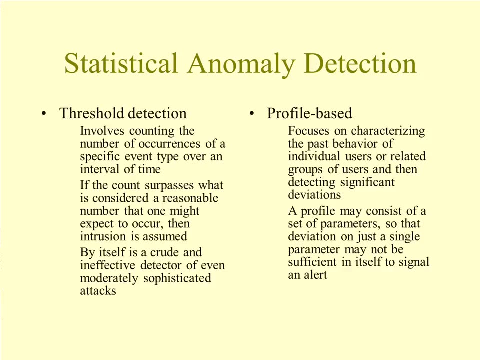 An advantage here is that it could be made vendor-independent and ported to a variety of systems. However, there's extra overhead in having two accounting packages running on a single machine. So our statistical anomaly detection: We talked about this a little bit on one of the previous slides. 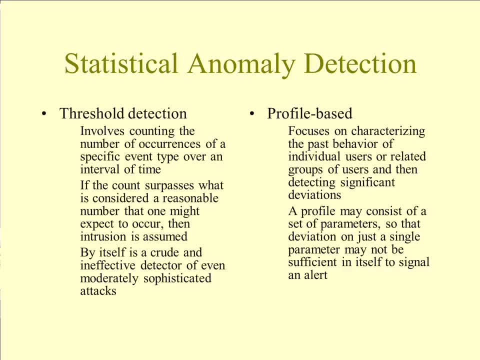 Okay, Let's go back to one of the previous slides. Threshold detection involves counting the number of occurrences of a specific event type over an interval of time. If, for some reason, that count surpasses what's considered a reasonable number, and the way that we can get this reasonable number is maybe by tracking this for legitimate users. 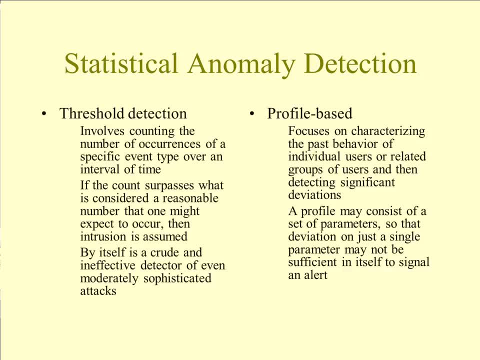 over a certain amount of time and finding out what's considered reasonable. So if it bypasses that, then we will say that maybe an intrusion is occurring and we can alert some network administrators So they can go check it out. By itself this is a crude and ineffective detector of even moderately sophisticated 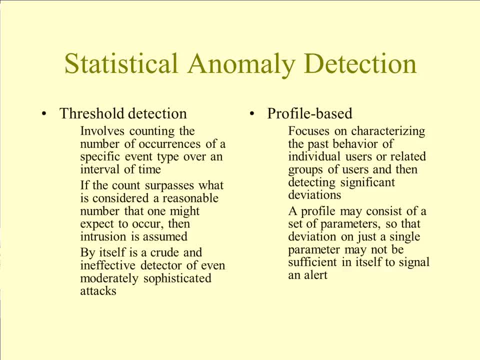 text. There are going to be a lot of false positives with this. Maybe somebody at lunchtime decides that they're going to get onto YouTube or that they're going to go onto eBay or something like that, and it might just be out of the norm and it's. 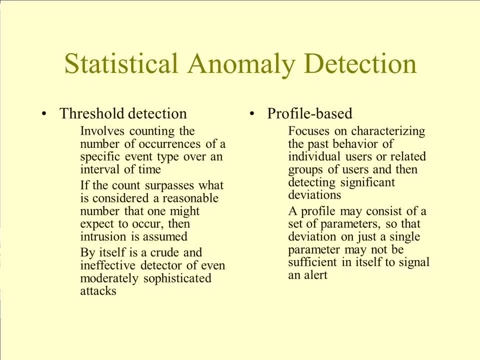 going to raise this red flag using threshold detection, or it's possible that it could With profile-based analysis Anomaly detection. It focuses on characterizing the past behavior of individual users or related groups of users and then detecting significant deviations. The profile may consist of a set of parameters so that deviation on just a single parameter. 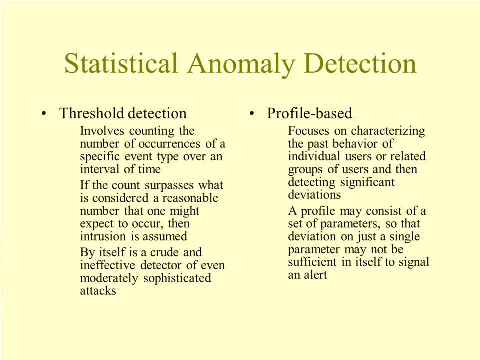 may not be sufficient in itself to signal an alert. The foundation for this is the analysis of the audit records that we just talked about. The audit records provide input to the intrusion detection system. The designer must decide, then, on a number of quantitative metrics that can be used to. 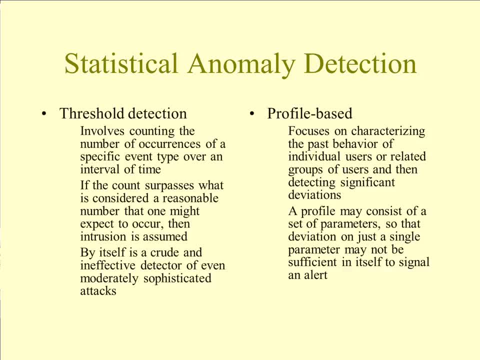 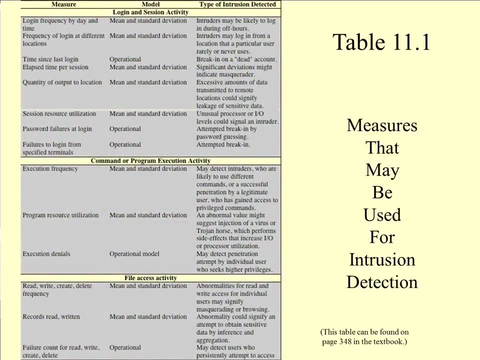 measure user behavior. The audit records then serve to define typical behavior, So the intrusion detection system then analyzes the incoming audit records and determines if there is some deviation from the average behavior. Here are some measures that may be used for intrusion detection, So this could be some of the things that you would see on that graph. 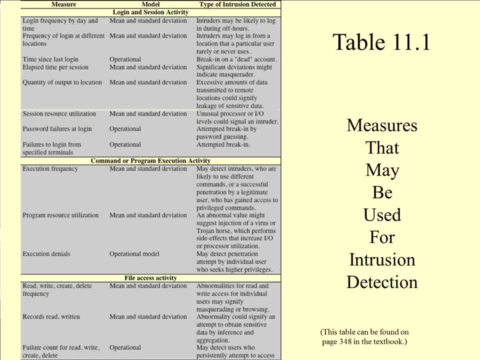 That we saw on one of the previous slides. Login frequency. location of login time since last login. elapsed time per session. quantity of output to the location. password failures: how many password failures are there at login? the frequency of execution of specific programs. resource utilization: denials of execution. 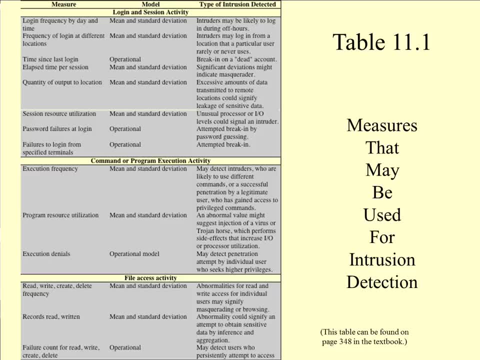 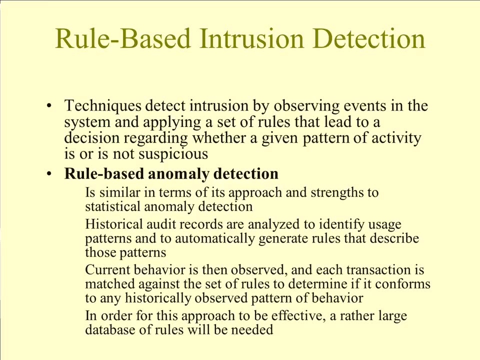 of a program, how much reading, writing, creating and deleting is occurring during that session. How many records are read and written. So these are some things that can be monitored so that you can try to detect if an intrusion is occurring. Rule based intrusion detection involves techniques that observe events in the system and apply 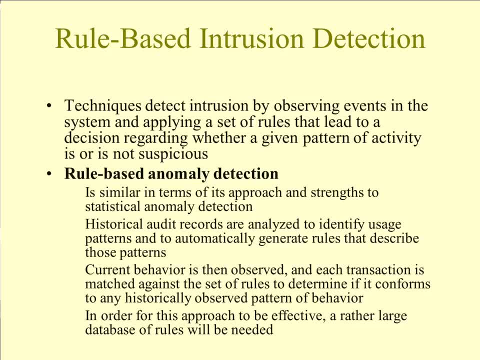 a set of rules leading to a decision regarding whether a given pattern of activity is or is not suspicious. So you can see down on my bottom bullet There. the rule based anomaly detection is similar in terms of its approach and strengths to the statistical anomaly detection. 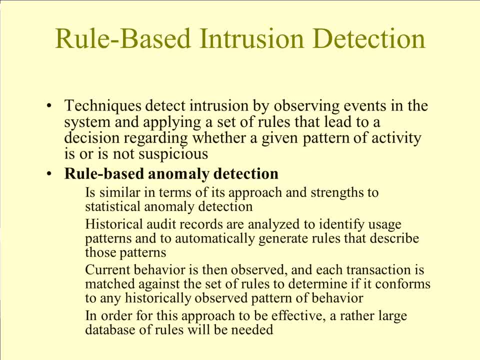 However, historical audit records are analyzed to identify usage patterns and to automatically generate rules that describe those patterns. So these rules may represent past behavior patterns of users as well as the current behavior. So it's a little bit more sophisticated. however, you have to have a little bit more data to 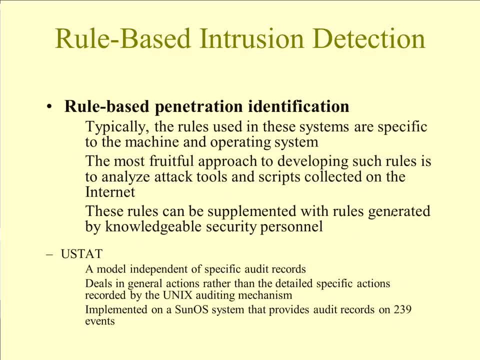 operate on. It might take a little bit longer for detecting Rule based penetration. identification takes a different approach to intrusion detection. The key feature here is the use of rules for identifying known penetrations or penetrations that would exploit known weaknesses. So this would be: if we know that we have some kind of an exploit or some kind of a weak. 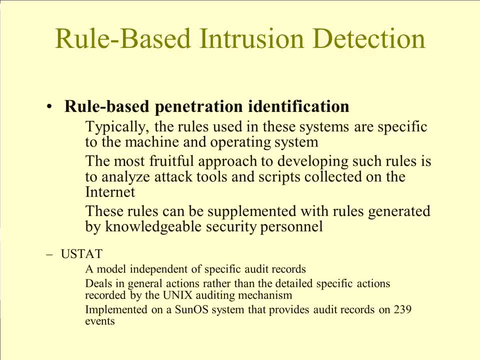 penetration somewhere, then the rules based penetration would probably be what we want to use. We have a server where we can't update it because it's going to break our current application, but we know that there is a security risk there, So we could do something like this with rule based intrusion detection to just try to monitor. 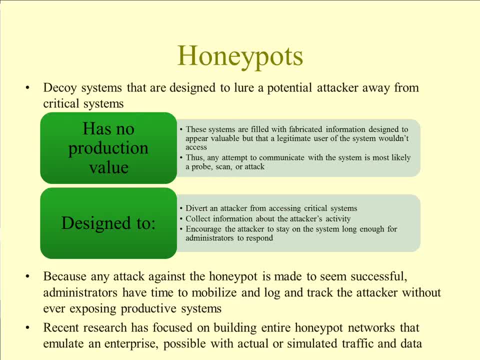 it and see if something is occurring. Honeypots are a really, really interesting innovation that we have as far as intrusion detection is concerned. Honeypots are just decoy systems. They're designed to lure a potential attacker away from critical systems. 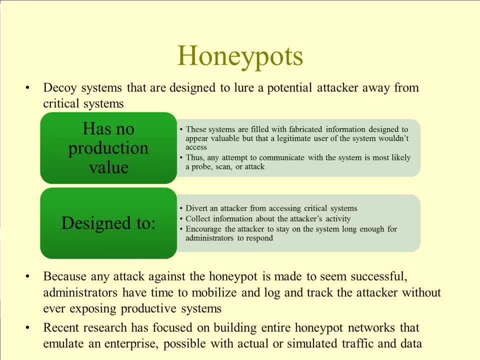 They're designed to divert an attacker from accessing the system, collect information about the attacker's activity and then encourage the attacker to stay on that system long enough for administrators to respond. This is really neat that we have this honeypot, which is sitting somewhere either on the network. 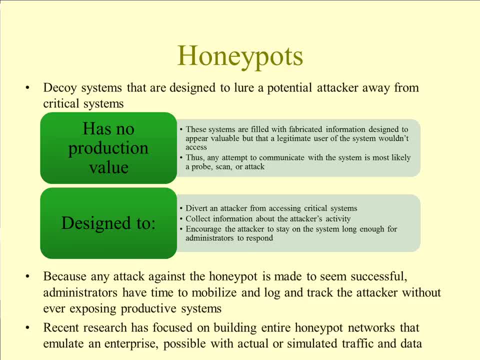 or just outside of the network And it's just there as a decoy, trying to get people to go to the honeypot rather than try to attack the systems that are inside. There could even be a data That seems to be legitimate there. 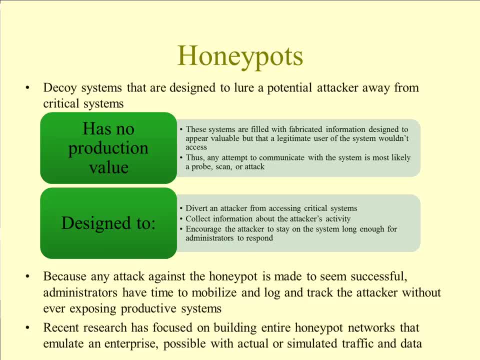 But legitimate users would know that there's a honeypot and not try to access that. So any access which is going on in the honeypot, you can assume is probably going to be an attack. So you can make the attack even seem successful, which is going to keep the attacker on that. 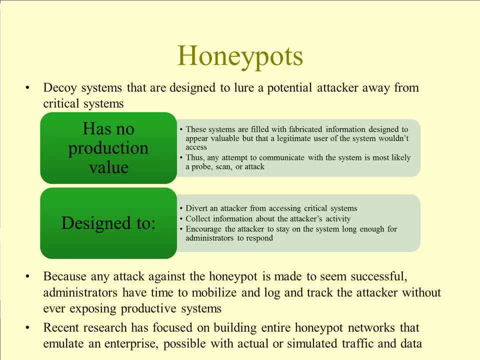 system longer so that you can try to track them and find out more about what they're doing. And there's a lot of work on honeypots And creating honeypots. right now that's going on And even creating entire networks of honeypots. 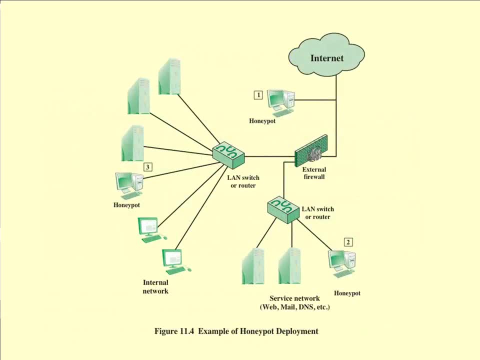 It's really interesting something that you should try to read about outside of this class also. Here's just one example of where a honeypot could be, So it could be outside of the external firewall even So. you try to block all the traffic that you possibly can coming through that firewall. 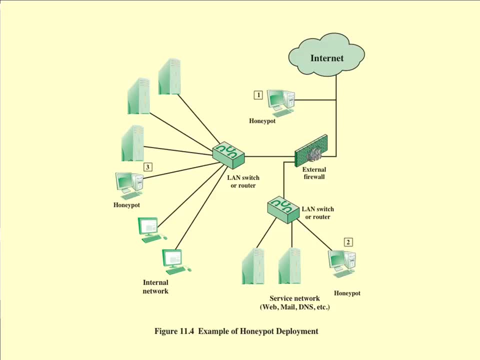 However, a user might think that they're accessing something inside the firewall if you have a honeypot sitting outside of it. So kind of a neat invention, A neat way of going about Trying to detect what's going on. So that's a neat way of going about trying to detect what's going on. 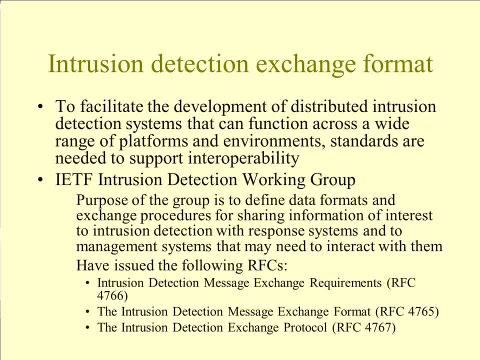 That's a neat way of going about trying to detect what's going on. So you can see here how we've been able to make some sort of data on the network. So to facilitate the development of distributed intrusion detection systems that can function along a wide range of platforms, standards are needed. 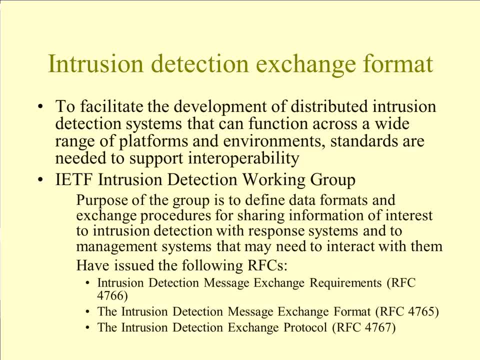 So the Internet Engineering Task Force, the IETF, has an intrusion detection working group, And what they're doing? the purpose of this group is to define data formats and exchange procedures for sharing information, And so, as we go along, you can see that there's a lot that's going on. 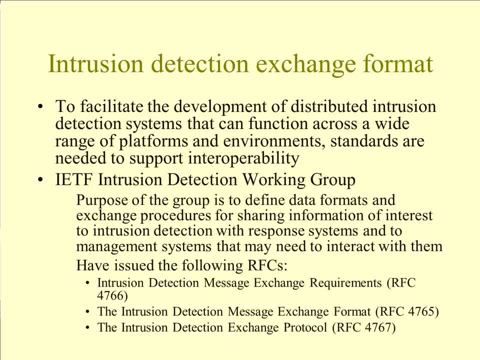 of interest to intrusion detection with response systems and the management systems that may need to interact with them. This is hopefully going to improve the intrusion detection systems that are already out there. There are some RFCs already: 4766,, 4765, and 4767,. 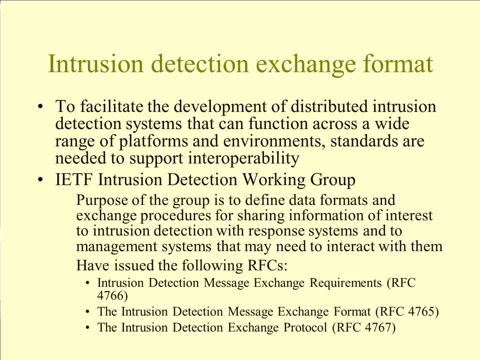 that define these Not very interesting reading. These were all issued in 2007.. So if you want to take a look at those, those would probably be helpful. if you really like intrusion detection systems and how they work, If you potentially want to work on one, 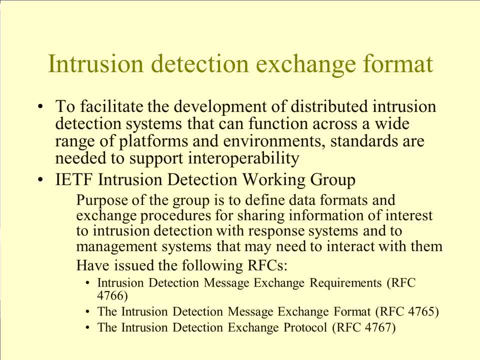 you probably are going to need to know what those RFCs are. Okay, so hopefully you enjoyed this lecture on intrusion detection systems. I would suggest that you go out, look up some intrusion detection systems, even install them on your computer. Try to get a little bit of experience with how they work.